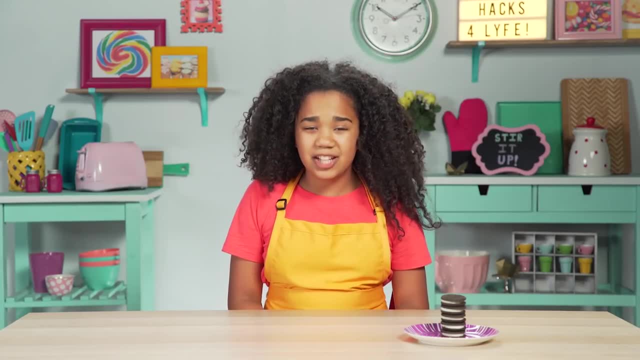 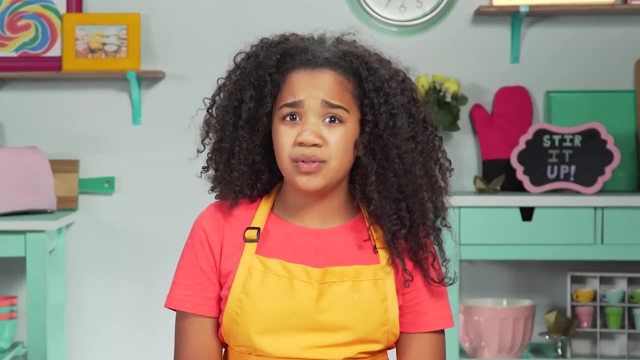 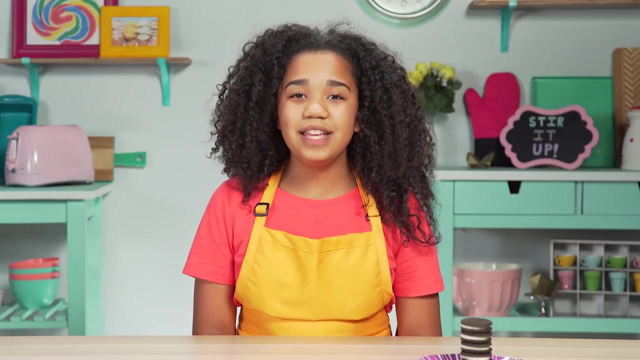 Hey guys, it's me, Whitley, and my love for Oreos is actually redonkulous. but after eating over a hundred thousand Oreos, they're turning into boreos. That's why today's hacks are Morioh Oreo Fusion Hacks. My first hack infuses Oreos with the cuisine of the east. Let's make. 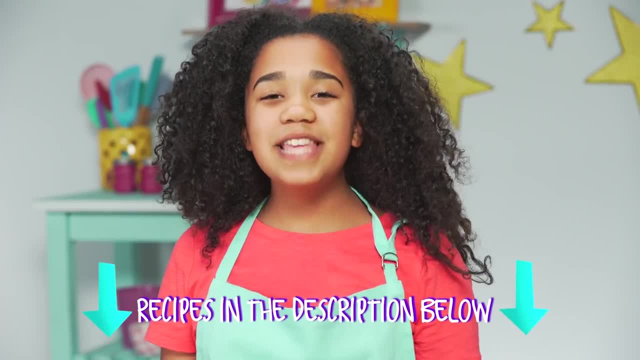 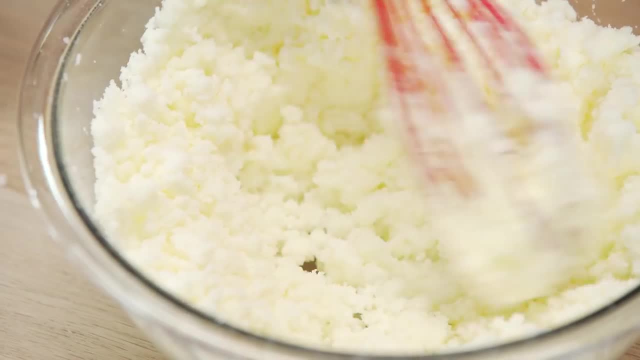 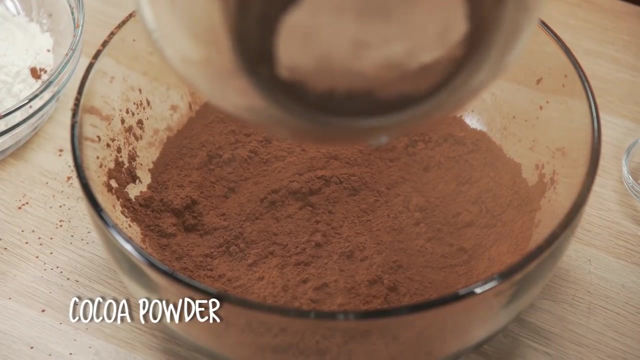 my crazy Oreo dumplings. All these hack recipes are in the description box down below. Combine butter and sugar in a bowl and mix it together. Add in your eggs and vanilla extract In a separate bowl. combine cocoa powder, flour and salt. 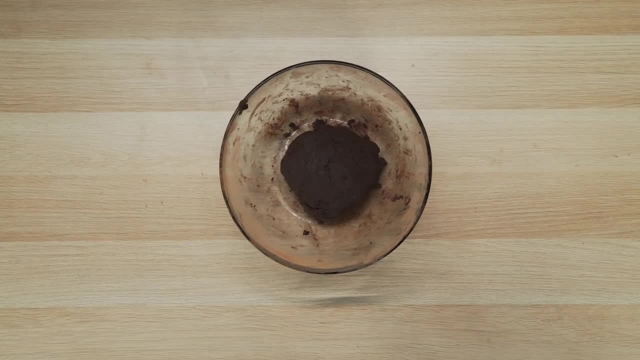 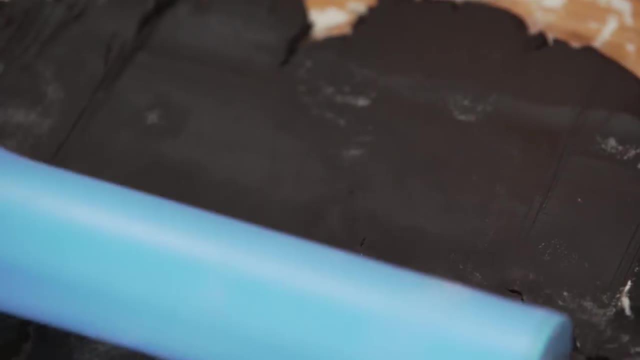 Mix it then knead it until it becomes dough. Wrap in plastic wrap and let it cool in the fridge for one to two hours. Roll out the dough with flour and cut out circles with a cookie cutter. Take more dough and place it in the middle of the circle. 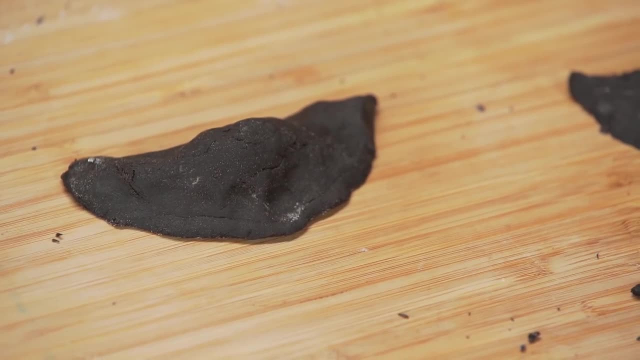 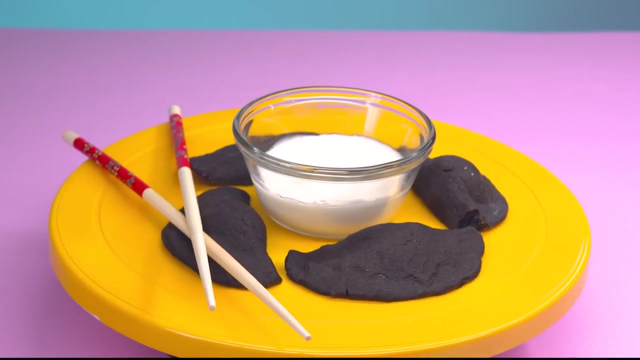 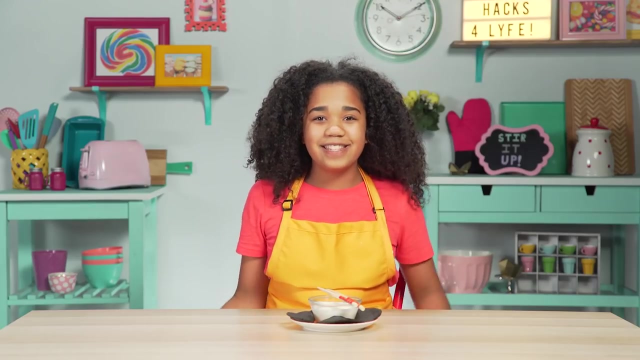 Close the cookie, Press it to seal it, shut, Shape it into a dumpling, Place on a baking sheet and bake at 325 degrees for 17 minutes. I can't believe these were Oreos and now they're dumplings. But before we dip our dumplings, 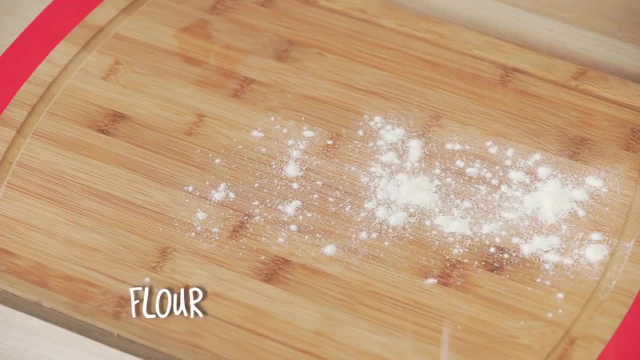 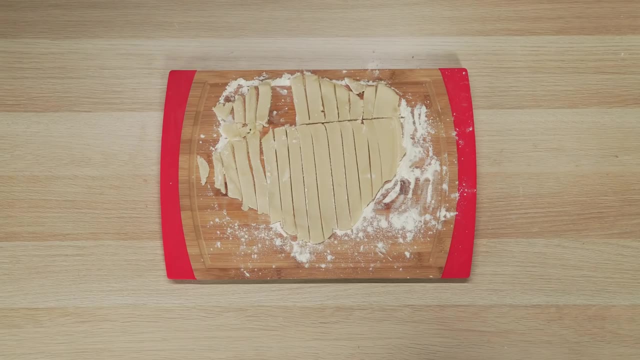 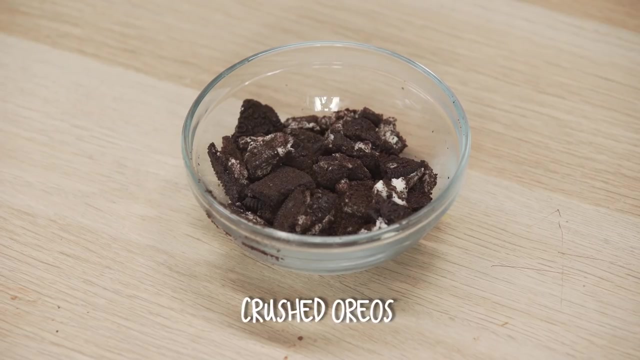 it's time to try my insane Oreo fries. Roll out your sugar cookie dough. Cut them into fry strips like this. The cookies will expand in the oven, but you can reshape them once they're out. Set aside a quarter cup of crushed Oreos. Melt chocolate candy melts in the microwave. 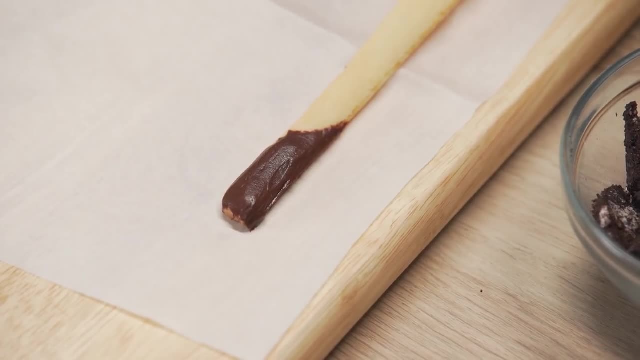 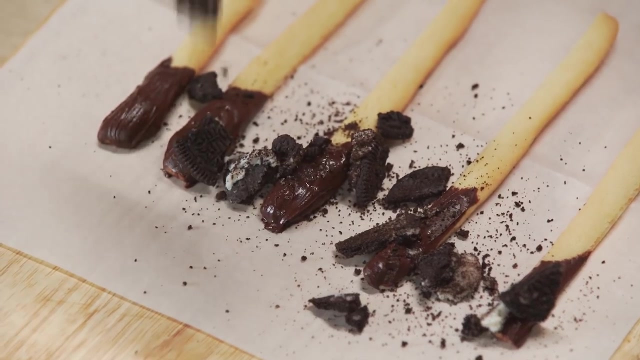 Dip the cookie fries into the chocolate and place them on parchment paper. Sprinkle crushed Oreos on top and let them cool in the fridge for five minutes. I can't believe these French fries were made out of cookie. I've only got hard ice for these fries. 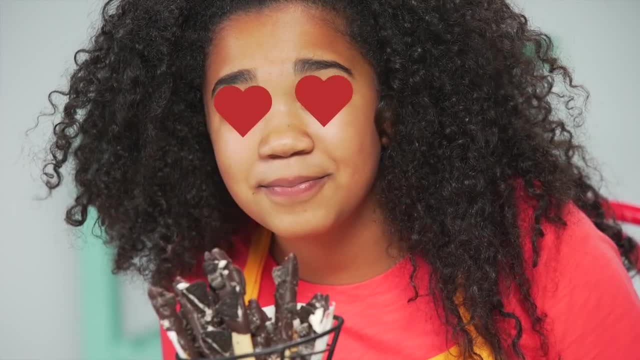 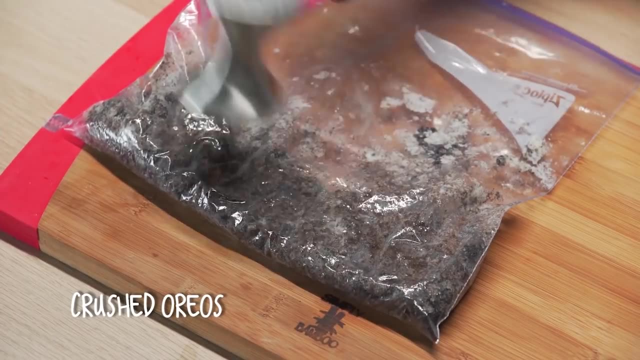 I also have hard ice for my last hack: my Oreo Ringo Pot. Crush your Oreos in a Ziploc bag. Now melt your white candy melts in the microwave. Mix in the Oreo crumbs. Grab your Ring Pop molds. Fill up with your Oreo mousse. 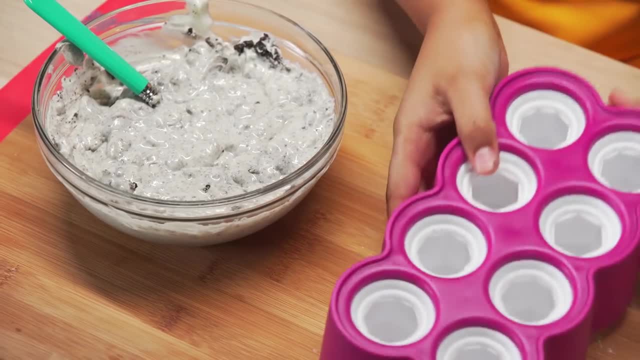